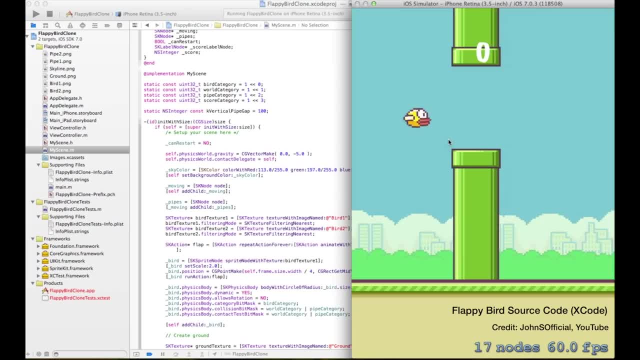 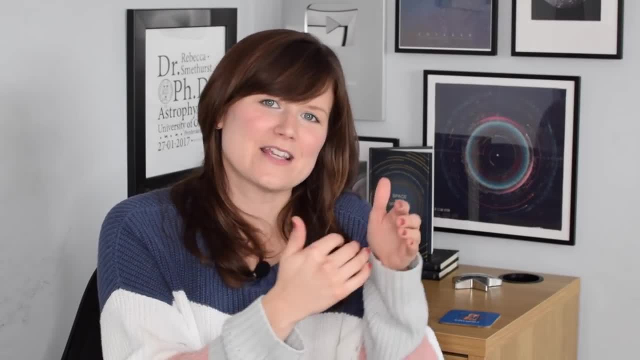 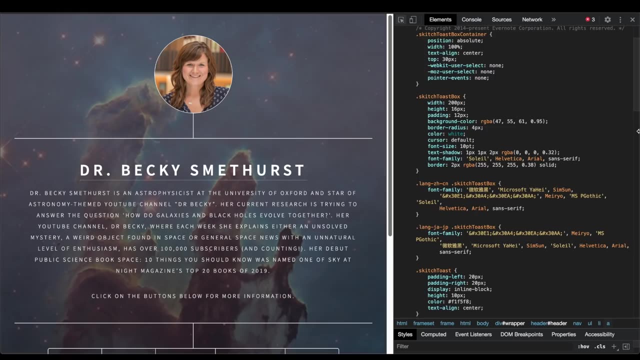 together, or how to format a web page, or even to designing a video game. All of these different tasks are best communicated to a computer with a specific language, usually a language that's defined for that set of tasks. For example, if you wanted to format a web page, you need a language. 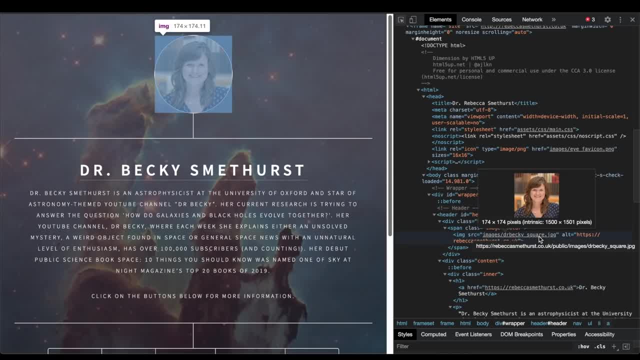 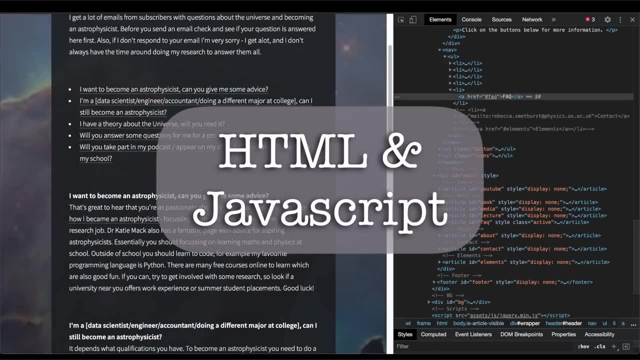 that would be a little bit more specific. So, for example, if you wanted to format a web page, you need a language that lets you tell it what font to use and how big to make an image on the page and what to do if people click on a specific button. To do that, people use HTML and programming. 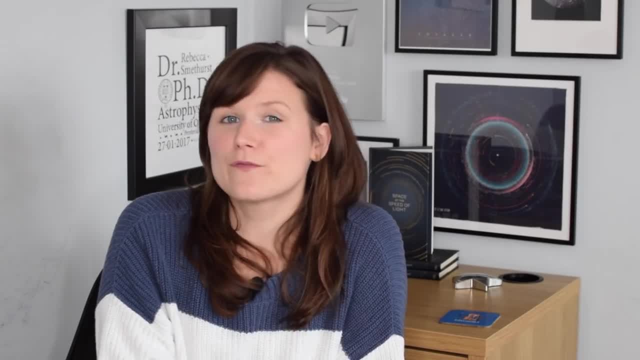 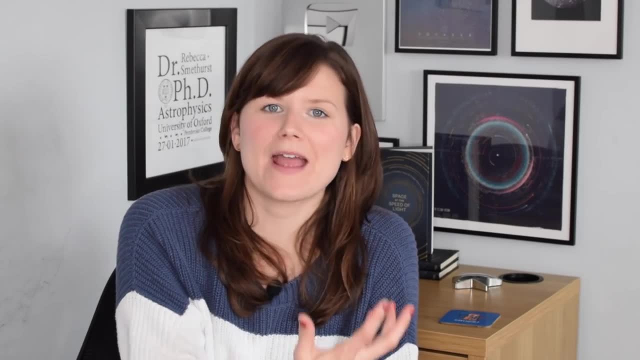 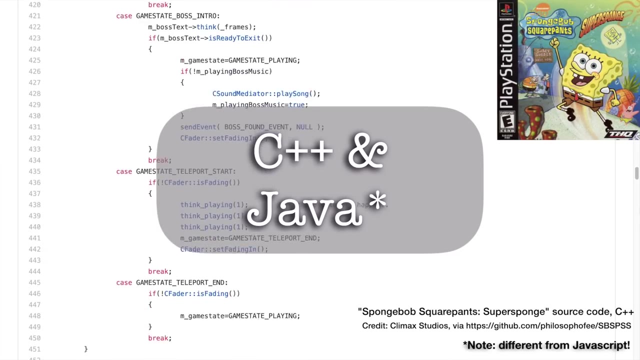 languages like JavaScript, Whereas for a video game, you want a language that's going to let you communicate to the computer how a character or an object behaves as you interact, as you play the game. So people use languages like C++ and Java to do that. 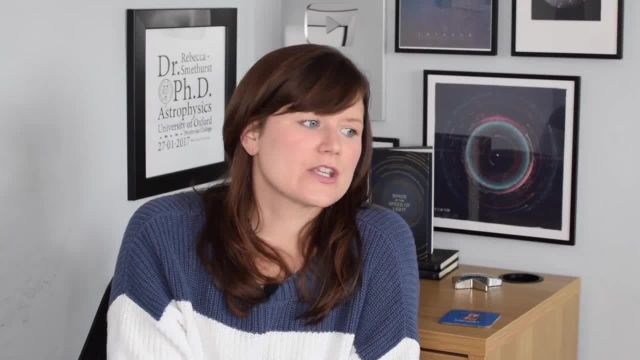 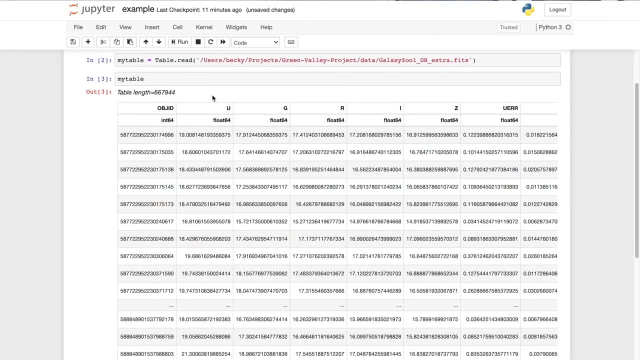 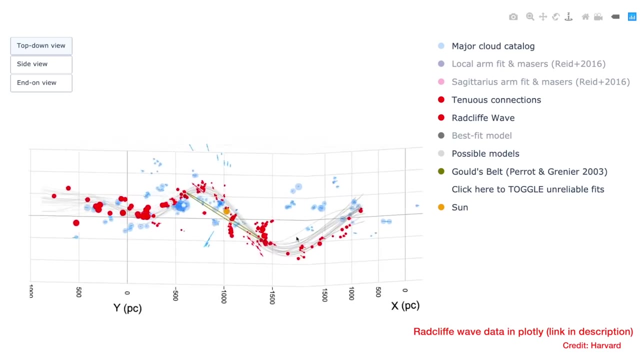 For science, though, it's a different story. You need a language that's both powerful and flexible, that's going to let you do things like read really large data tables or make plots to visualize that data or fit models to that data, Sometimes performing the same task over. 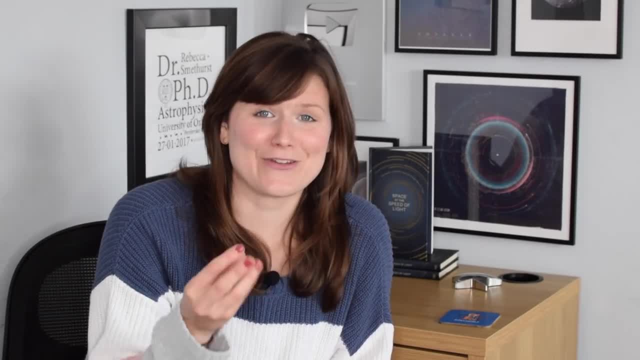 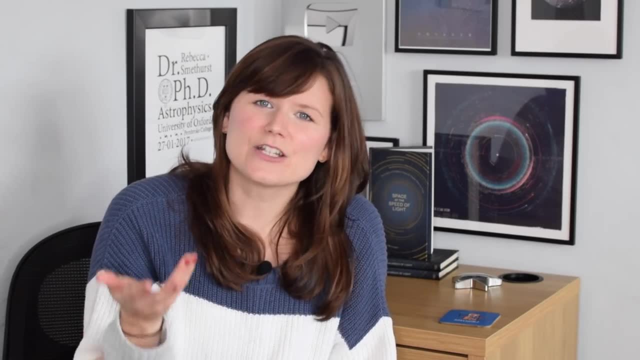 and over again, thousands, if not millions of times, and ideally you want it to do that in seconds, or at least as fast as it can anyway. Now there's a couple of languages that can do this, that are both powerful enough, flexible enough, but the easiest to read of those, and therefore 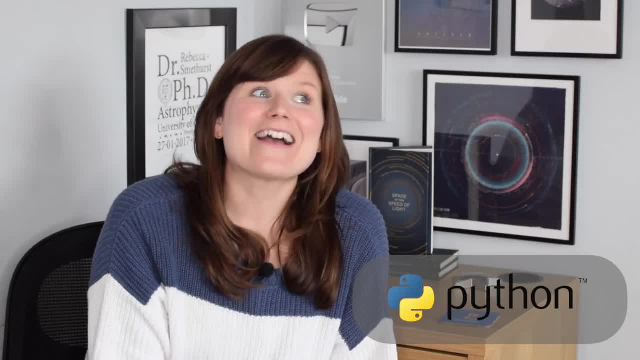 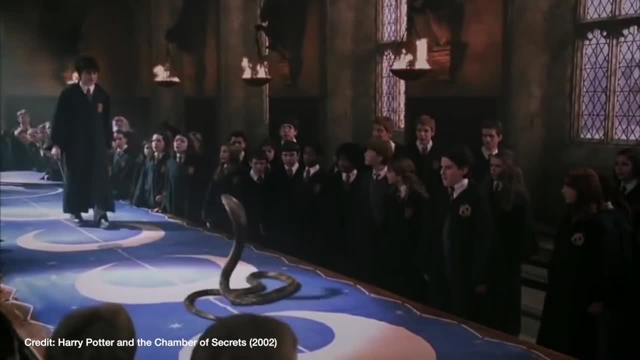 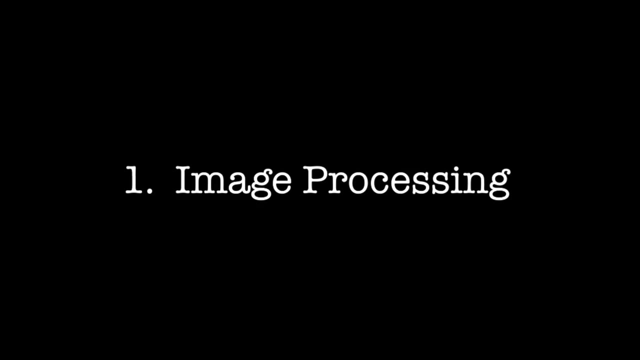 the most popular currently as well is Python, And that is my language of choice as well. I like to say I'm a Parseltongue and I use Python daily for doing my list of five things, So let's dive into this and start with number one: image processing. 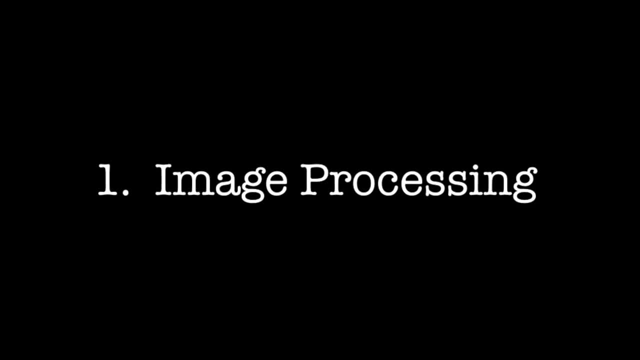 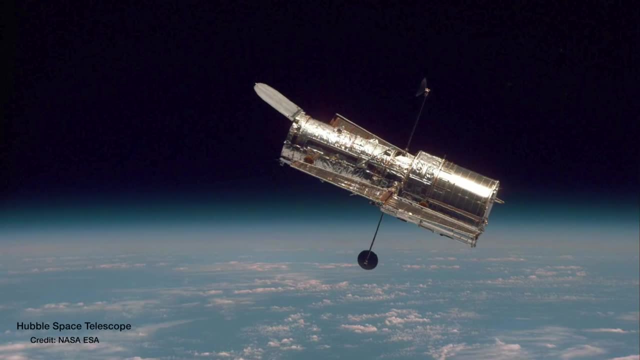 Now the first thing any scientist needs to do some science is data, and in my case, it's an astrophysicist. that data is images of galaxies from telescopes, whether they be on the ground or in space. But there's lots of sources of noise in these images, and what I mean by noise is light. 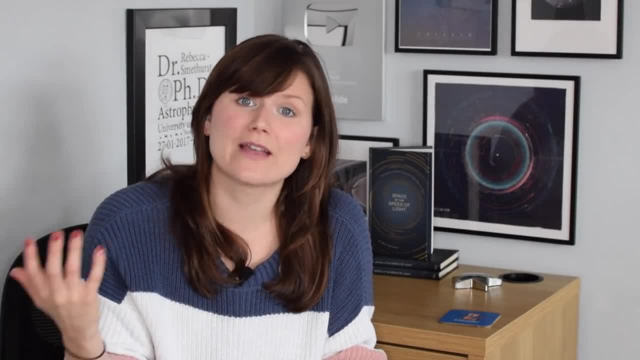 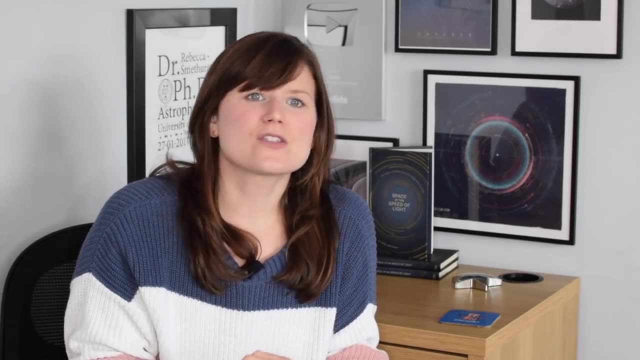 not from the object you care about, but from some other source that you don't care about, Whether that might be background noise from the sky itself, with just light bouncing around the atmosphere, or whether it's noise in the detector. So if you just left the shutter closed and you kept the detector, dark and still took an expression, you're going to get a lot of noise. So if you just left the shutter closed and you kept the detector dark and still took an expression, you're going to get a lot of noise. So if you just left the shutter closed and you kept the detector dark and still took an, expression, you're going to get a lot of noise. So if you just left the shutter closed and you kept the detector dark and still took an expression, you're going to get a lot of noise. So if you just left the shutter closed and you kept the detector dark and still took an expression, you're going to 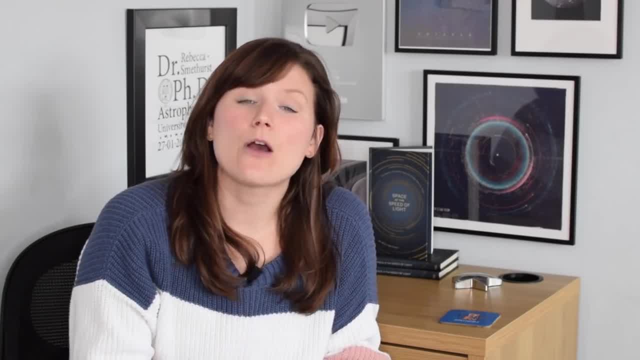 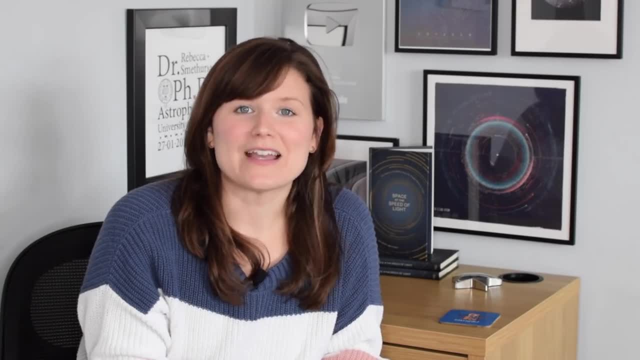 get a lot of noise. All of these sources of noise need to be accounted for and removed from your image so that you can do science with it. Essentially, you do that pixel by pixel, which is an incredibly tedious task, but it's one that a computer can do in seconds. 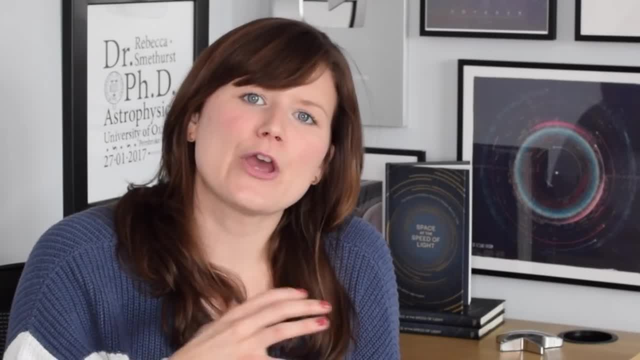 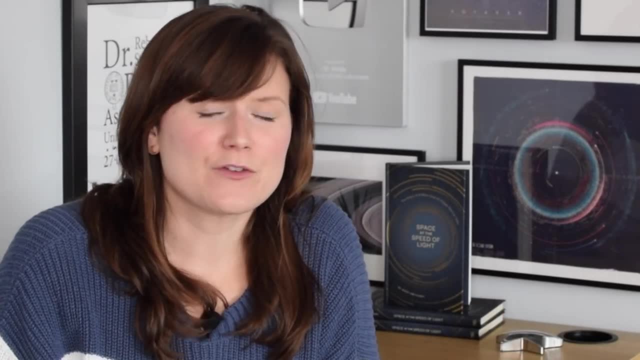 as long as you give it the right commands. Python is a perfect language for this, because one of its many strengths is being able to deal with big arrays of numbers. And what is an image, after all, but a big array of numbers, with each number telling you? 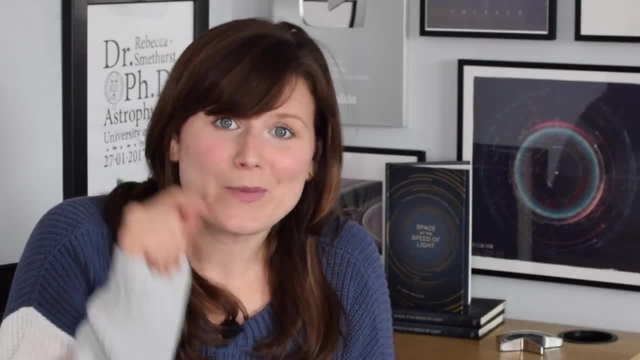 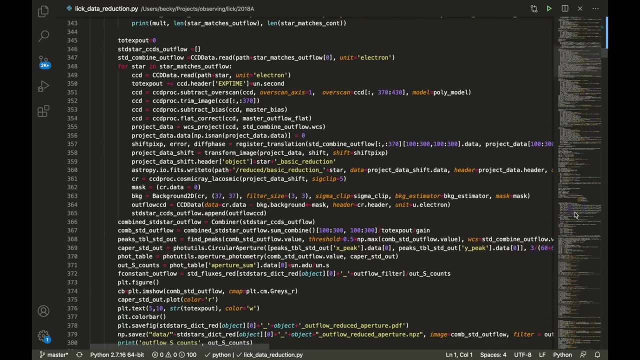 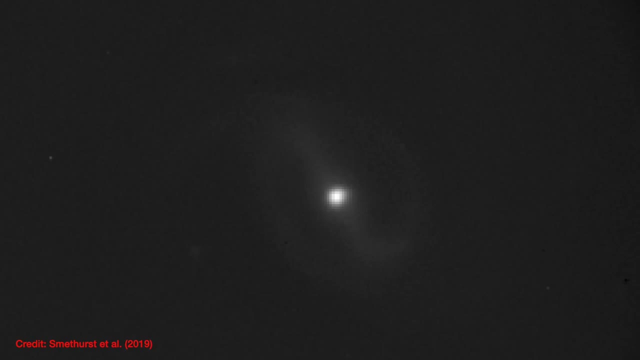 how much light has been detected in each pixel. With code like this, which is Python, using a lot of the AstroPy functions- an open source library of lots of coding functions- to do astronomically related tasks, you can turn messy, fresh off the telescope images like this into useful scientific 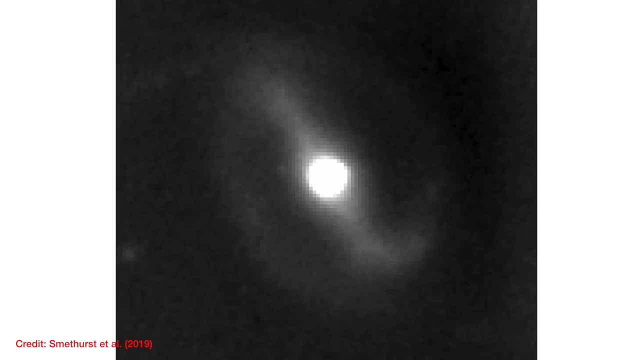 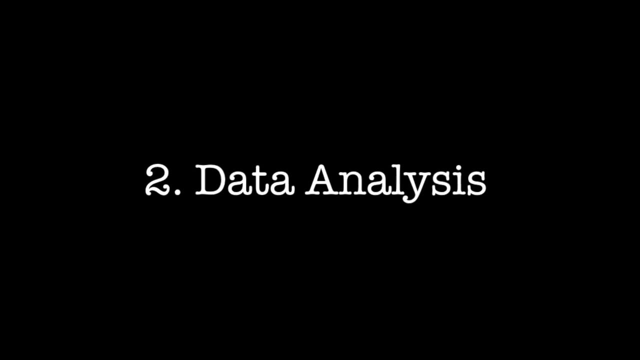 images like this, with only the light from the thing you actually care about left in the image. The second thing I use code for is data analysis. So once you have your scientific image of an object, in my case a galaxy, you might want to do some measurements on that image. 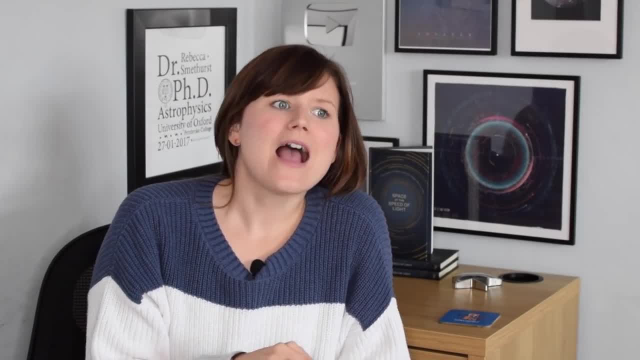 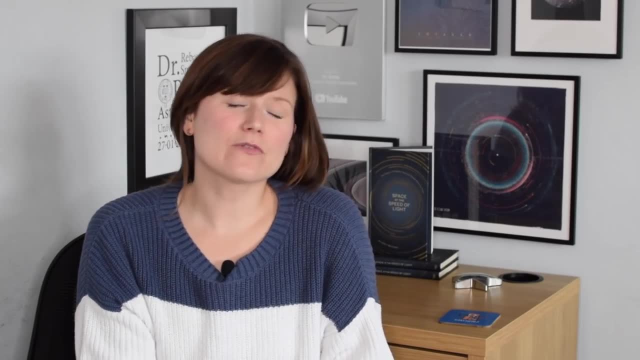 So you might want to measure how big the galaxy is, or how much light you've received from that galaxy in total, like how bright it is, or you might want to record how bright the central region is compared to the outside region, or the colour, and so on, and so on, and so on. 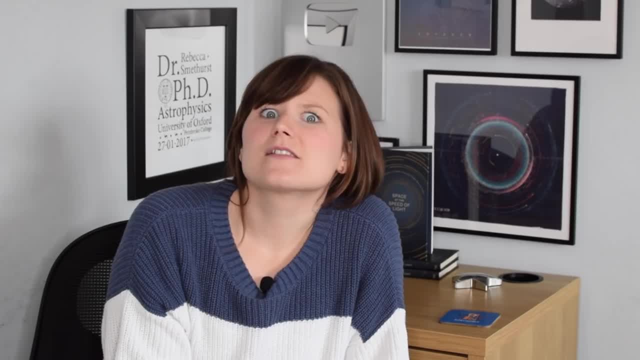 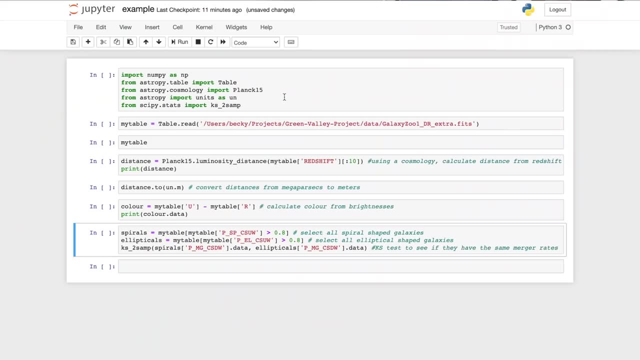 And if you do that for tens of galaxies, ten thousand galaxies, billion galaxies, you're essentially going to end up with a huge big data table of properties that you've measured. One of the longest data tables I have is over 600,000 rows long, That's. 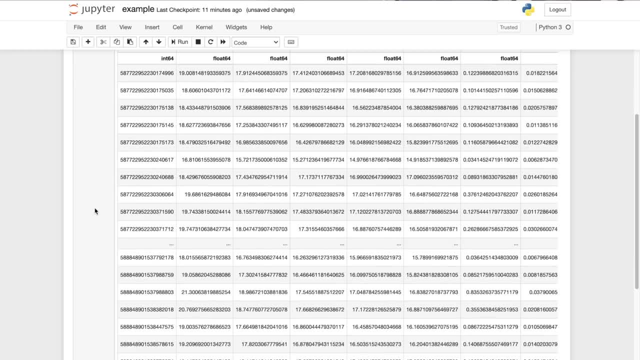 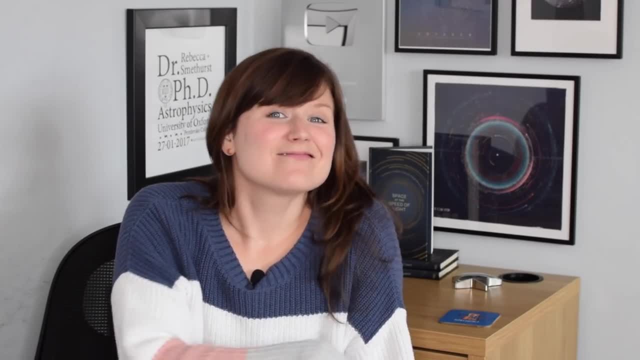 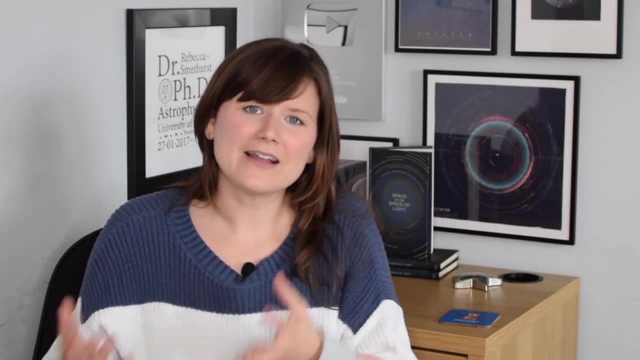 600,000 galaxies, each with different properties measured, That's far too long for any Excel spreadsheet to be able to handle. But again, Python is perfect for this, because this is just another form of an array of numbers, And so I can use Python. 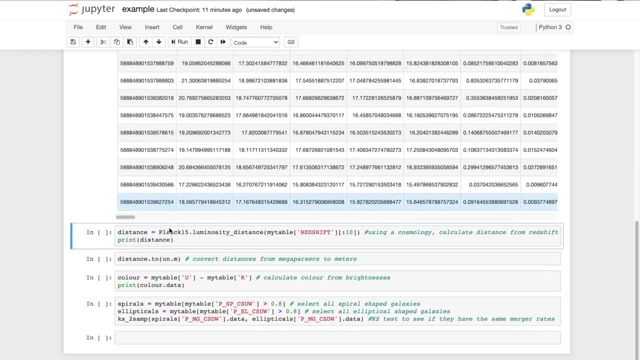 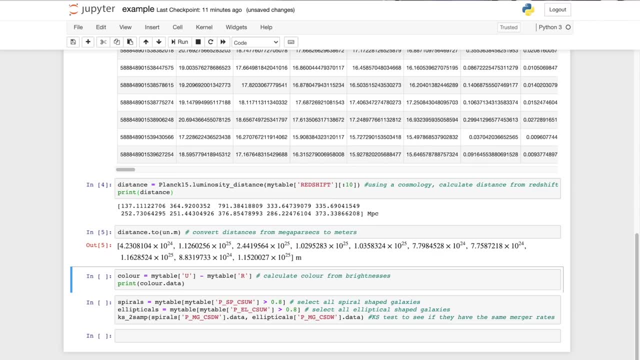 to play around with my data in this table. So, for example, for every single row in this table, I might want to convert one of the measured properties in a column into another unit, or I might want to use it to calculate another property, or I might want to do some statistics. 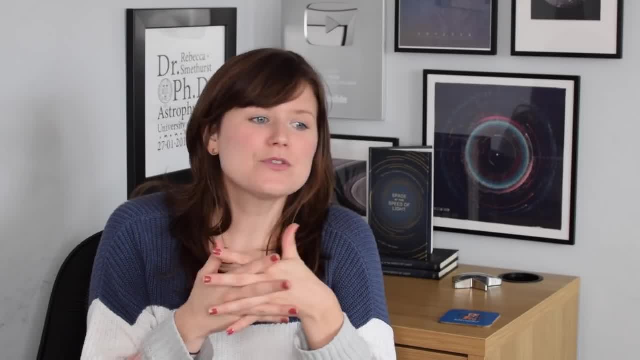 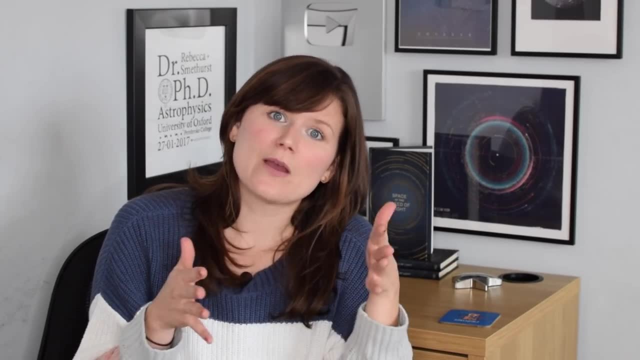 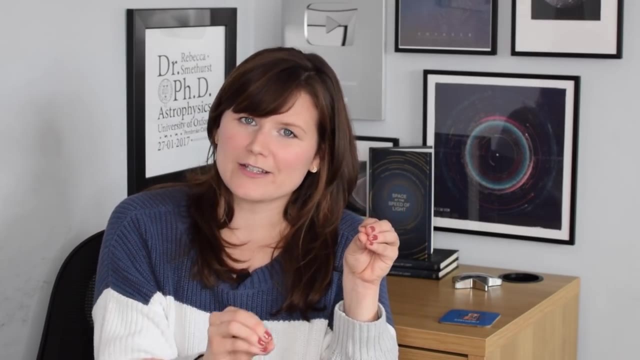 on my sample. Either way, given the right commands, a computer can do all of this on every single row in your data table, far quicker than either you or I would ever be able to do it by hand. Or you might want to do this by splitting your data table into chunks on an Excel spreadsheet. 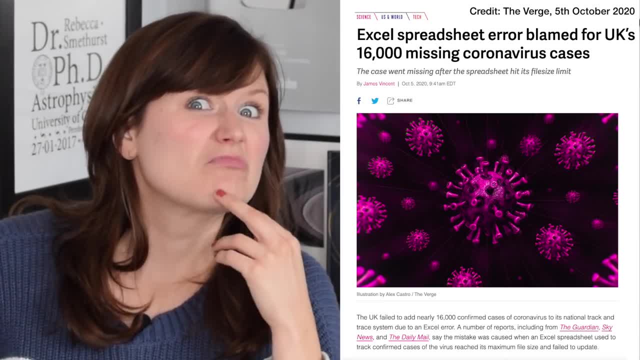 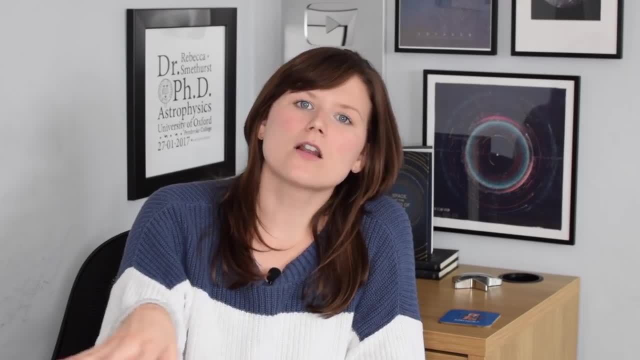 Someone might want to tell the UK government to track and trace people, that though Number three model fitting. So once you've got all of this data, you want to be able to understand the underlying physics of what's going on so that you can do some science. 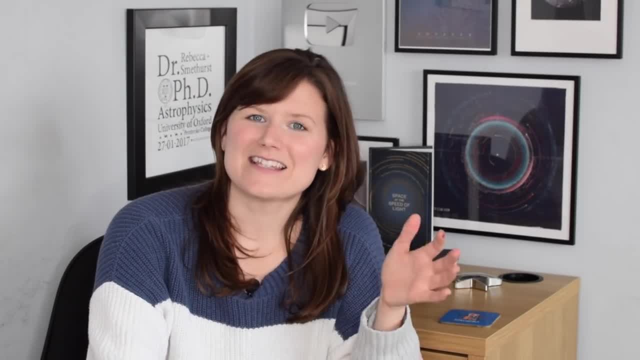 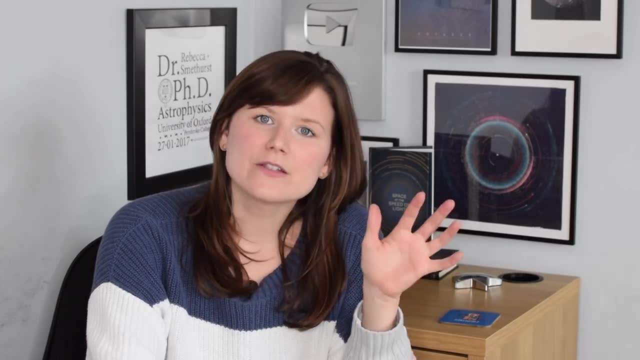 And one of the best ways to do that is actually to fit a model to your data. The best fit model can actually tell you a lot. It can tell you whether your assumptions about what physics is driving the results of your data are the right ones or the wrong ones. So you might want to. 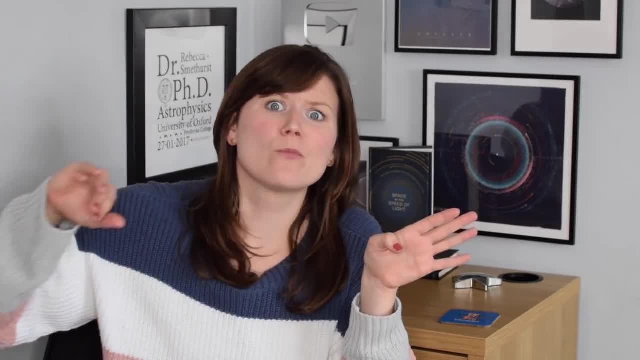 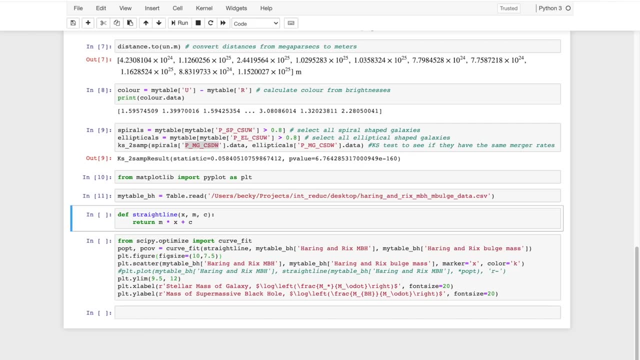 look at the results you're getting at actually right or not. Instead, if you have a terrible model, then you know that that idea was definitely wrong because it doesn't fit the data at all. The simplest form of that that people I'm sure will have come across is fitting a straight line. 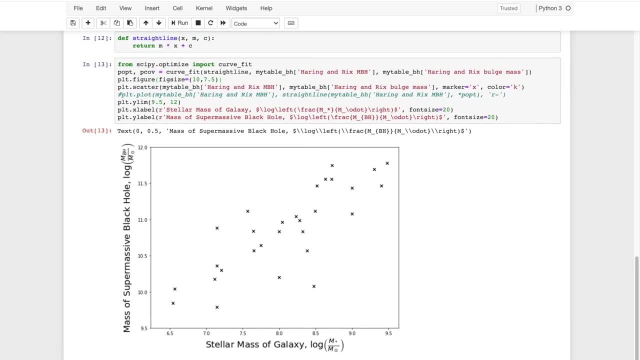 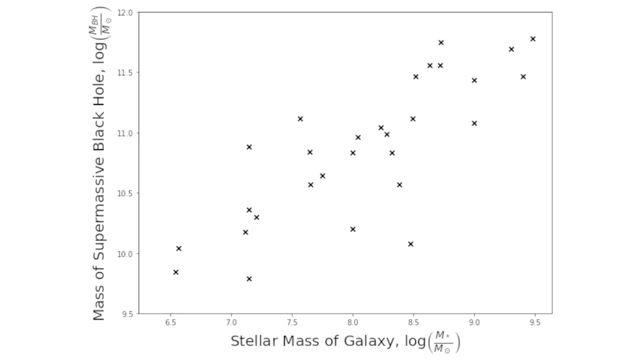 to some data. It's just a test of whether two properties are correlated or not. For example, here I'm showing the mass of a galaxy supermassive black hole and its overall mass in stars. You can see there's quite a lot of scatter, but it is still correlated And that led to the 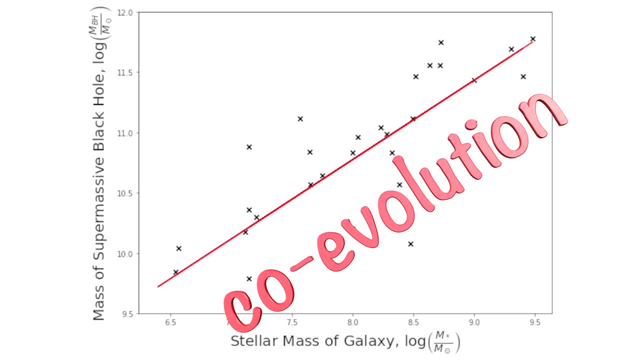 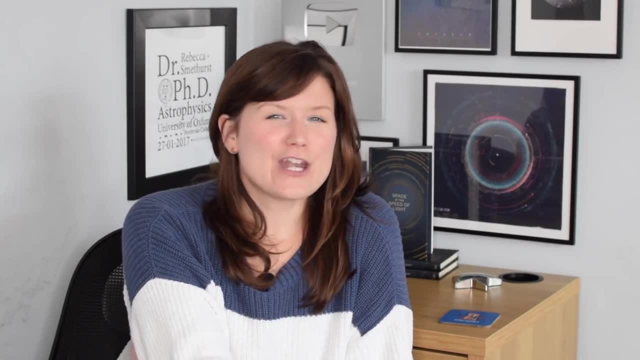 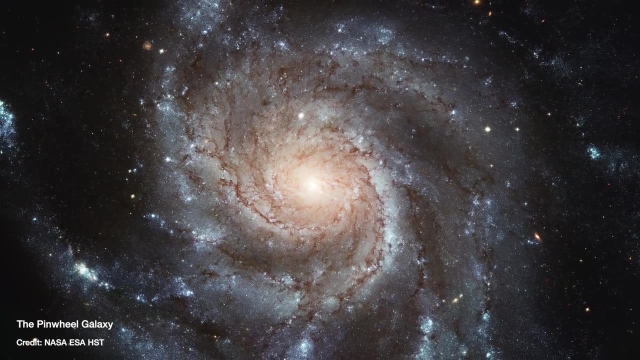 hypothesis that galaxies and black holes co-evolve and grow in mass together. But another thing you might want to do in terms of model fitting is infer an unknown from something you do know. For example, if a galaxy is very blue in colour, it has a lot of hot. 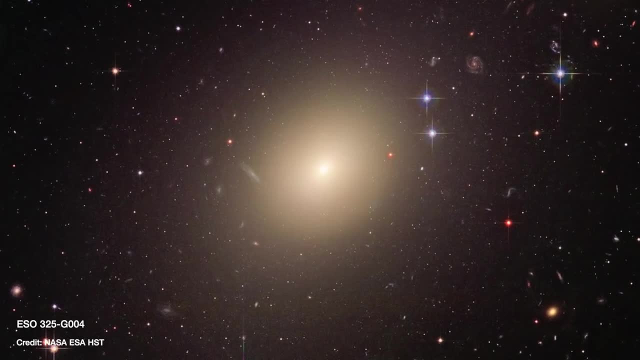 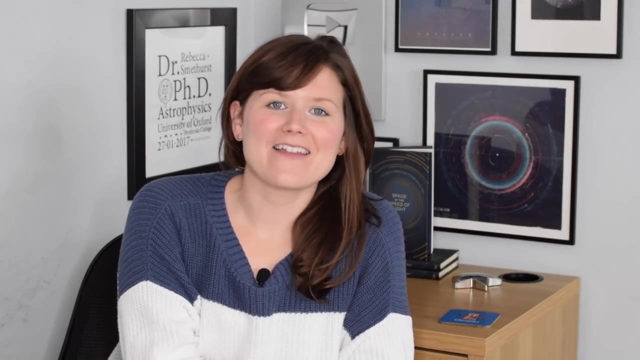 young big stars. But if a galaxy is very reddish in colour, it probably has a lot of old, cooler, smaller stars. I can then use those colours to ask: has that galaxy stopped forming stars recently? I do this by modelling the number of stars. a galaxy formed as an 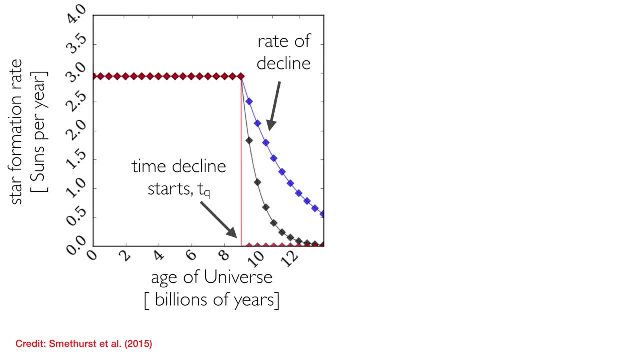 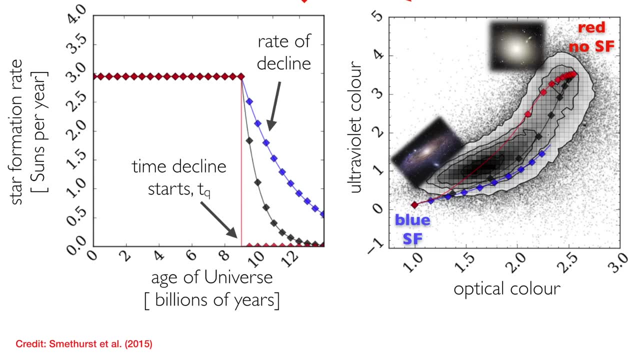 exponential decline of various different rates. I can then turn that into model colours, knowing what we know about how different masses of stars are different colours, And then I can say, okay, well, which model best fits the observed colour? I have in this image of the 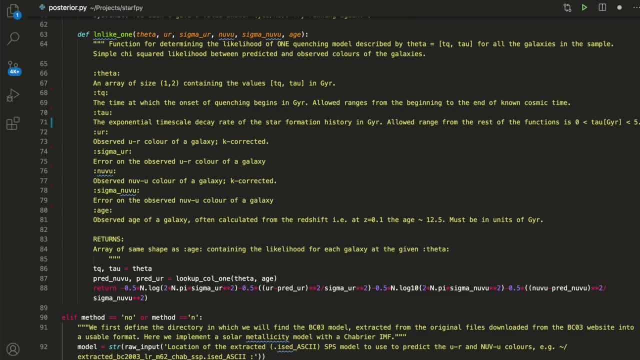 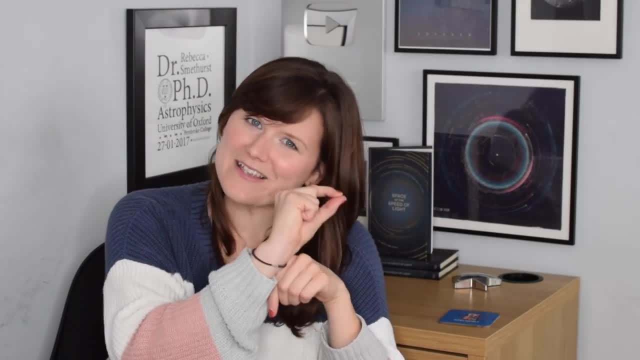 galaxy. I took So again, with some well-placed Python commands, this time just to find the minimum of an equation, ie when the difference between the modelled and the observed colours is the smallest it can be. you can find your best fit model and then off you toddle and do some. 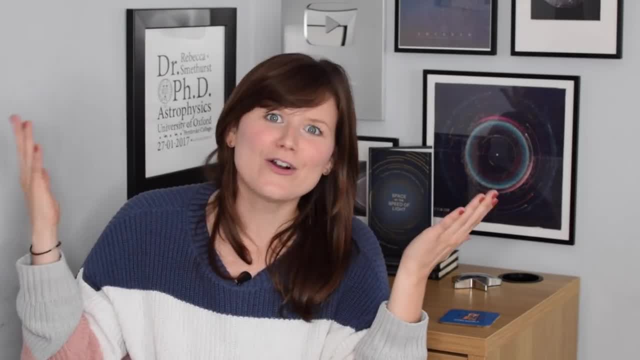 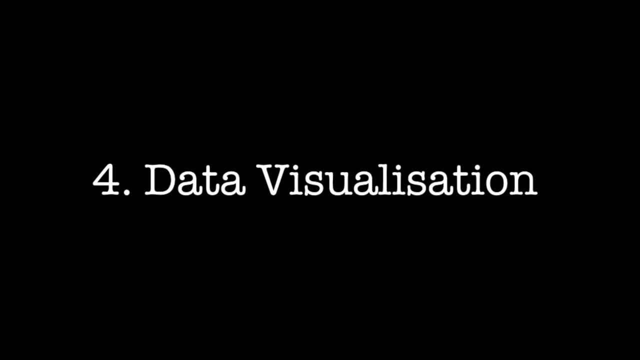 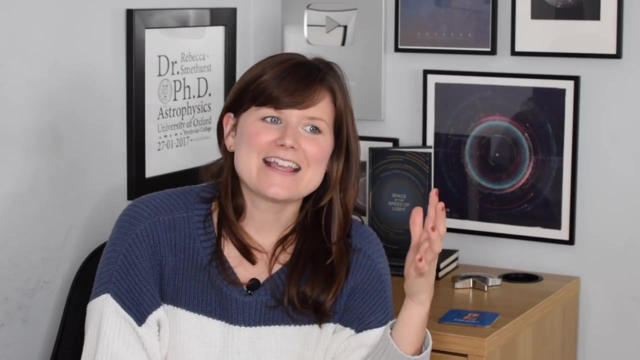 science and make some conclusions about what's going on in the universe. Number four: data visualisation. Now, once you've done all this data analysis and model fitting, you really need to be able to interpret all that information, And one way of doing that is actually. 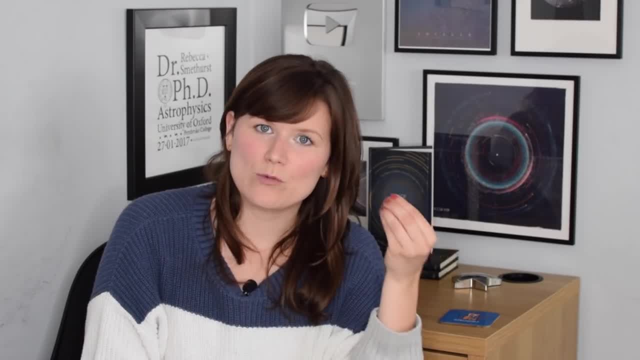 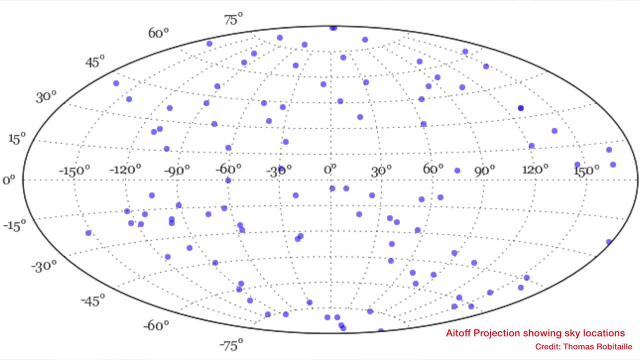 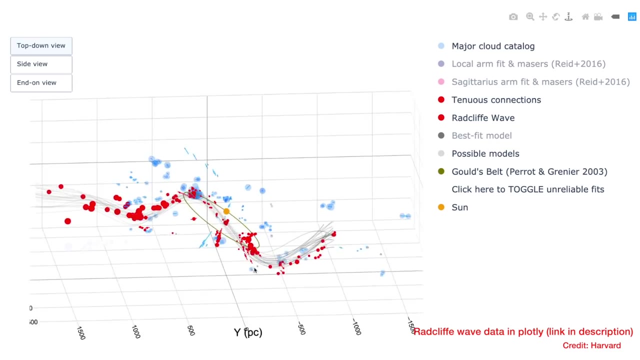 to be able to see your data and visualise more clearly what's going on, Whether that's with a simple histogram of the spread of a certain measurement in your data, or the location of objects on the sky, or even interactive graphics that you can play around with to see relationships. 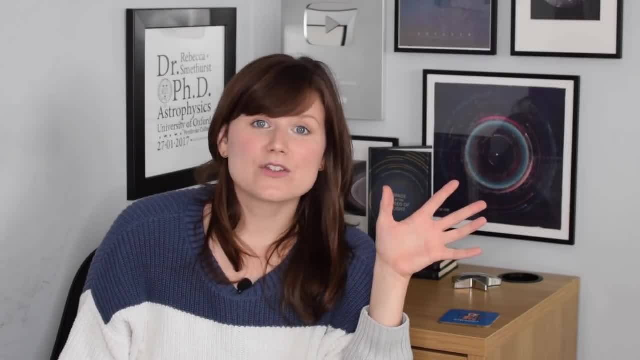 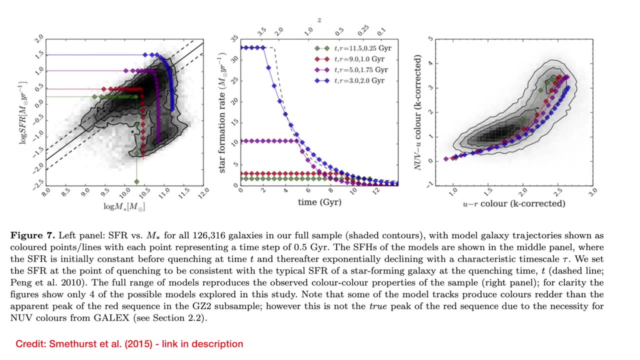 more clearly in your data. A few well-placed commands to your computer in Python and you can make some of the most beautiful scientific plots that will one day hopefully get published in a scientific research paper. Now the fifth thing in my list is simulations. This is when you code up. 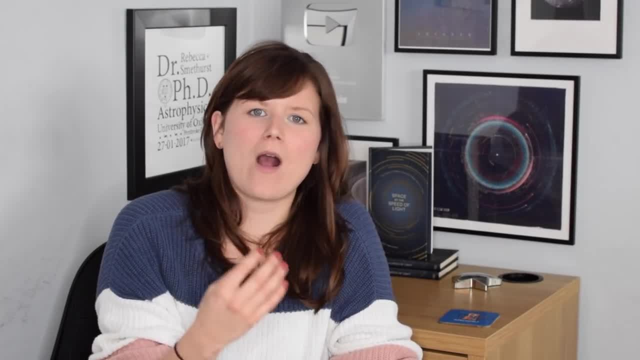 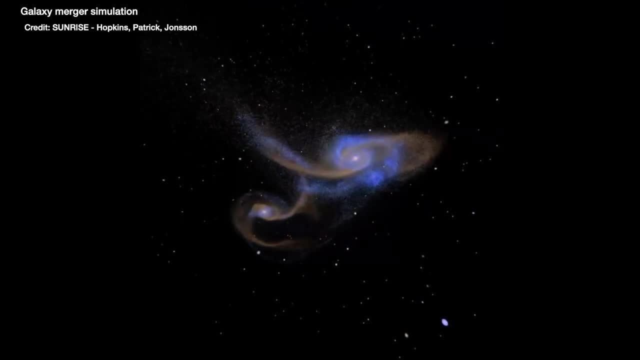 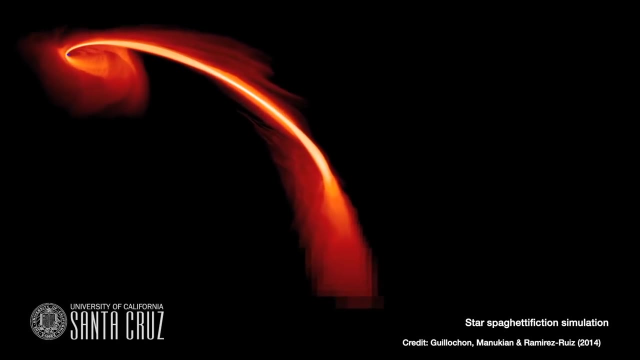 a program and run that program to try and recreate what happens when planets form around stars or what happens when galaxies collide, or maybe even what happens when a star gets too close to a black hole and gets spaghettified Unsurprisingly. that is incredibly complex. 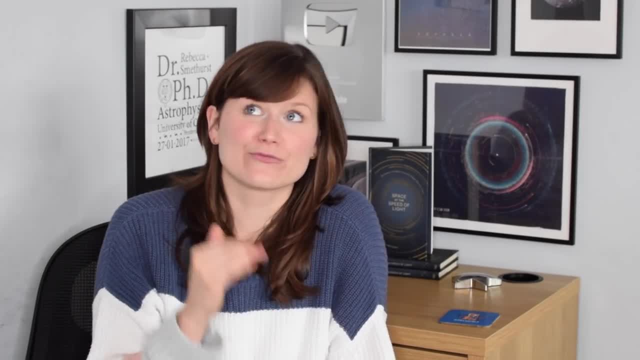 and it's something you have to dedicate your entire career to doing. I didn't do that because I wanted to use telescopes and look at real images of the stars and see what they're like. And I wanted to use telescopes and look at real images of the stars and see what they're like And 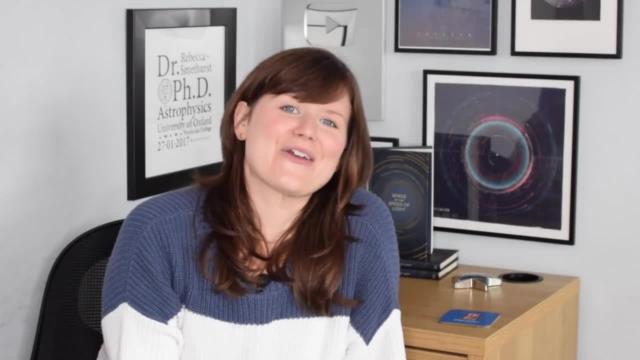 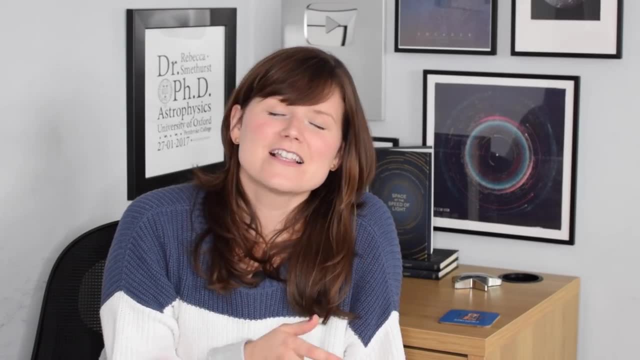 And I wanted to use telescopes and look at real images of the stars and see what they're like And galaxies in the universe. Someone who did do that, though, is one of my best friends from my PhD, Dr Ricarda Beckman, who is now a research fellow at the University of Cambridge. 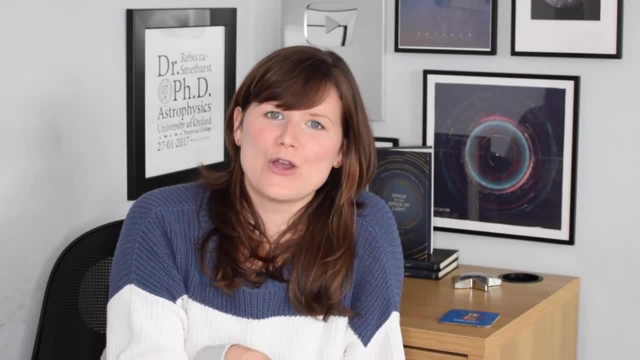 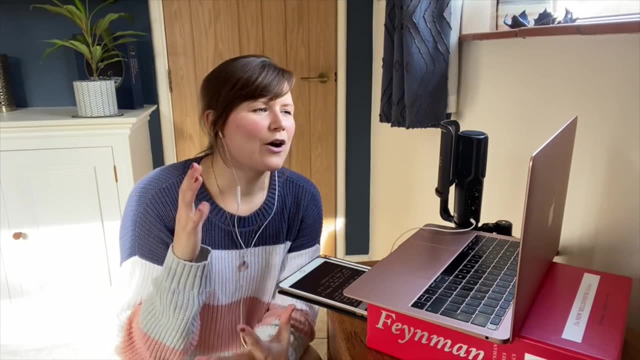 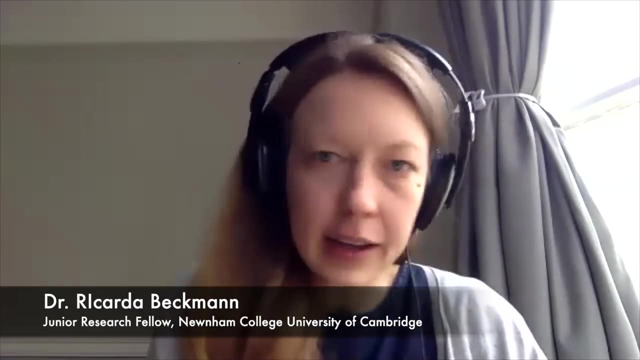 specialising in simulating how black holes grow. I rang her up to chat about how she uses code in her work. So how do you go about coding up something as complex as a black hole? So if you want to do a simulation of pretty much anything like a black hole or a galaxy or any other, 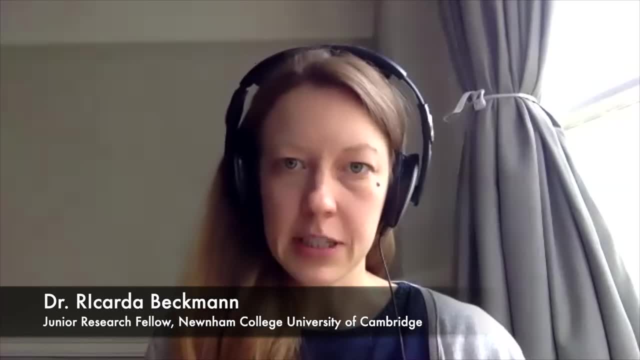 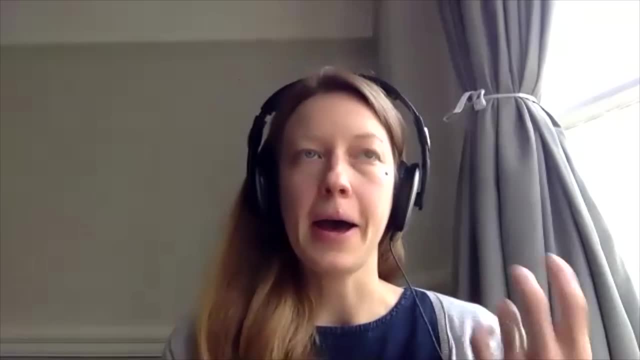 phenomenon. the key thing to think about really is the underlying physics. So we very much have to think back to sort of the parts or the components of physics that are relevant in this particular context, And then we think about how to translate the physical laws into some sort of computer. 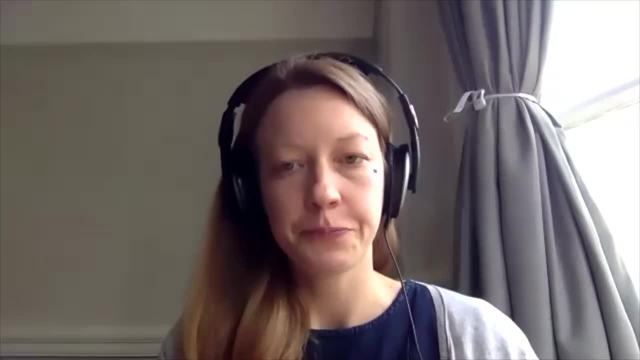 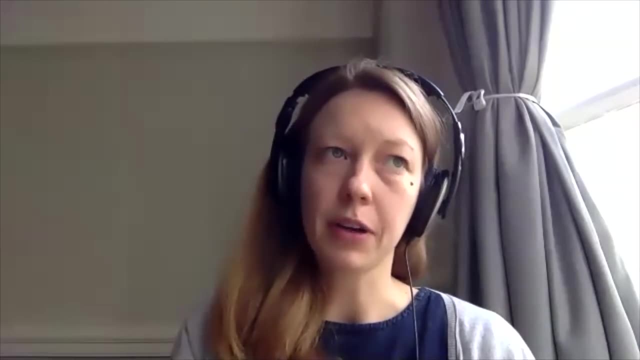 algorithms. So, for example, if I work with black holes a lot and I want to study, say, the evolution of gas near a black hole, what I'll do is I'll have to think about the gas physics. So I have to think about: OK, how does a gas behave, say, when the pressure changes, If you cool it or if you heat? 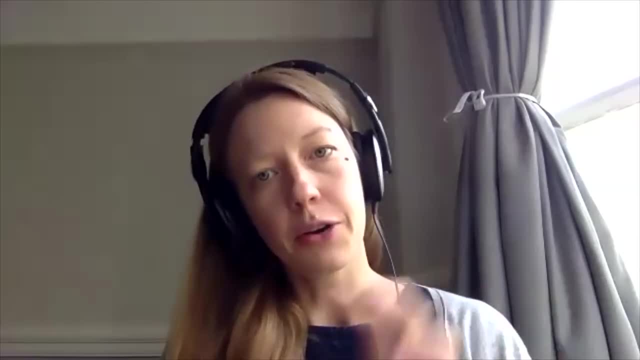 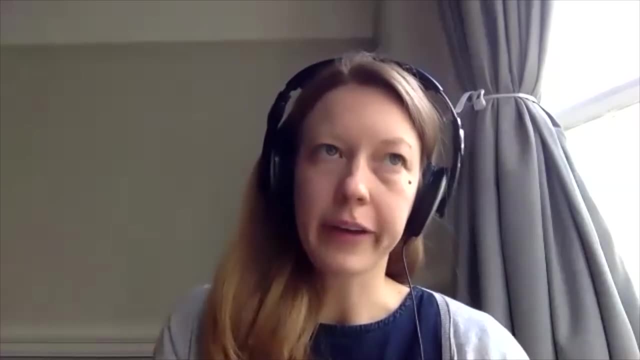 it? how does it move and evolve over time? So I will code up all these different sort of reactions on physical phenomena that go on at the same time, And then I have to think about the black hole and go: OK, so what does the black hole contribute to the situation? And for example, with black holes, 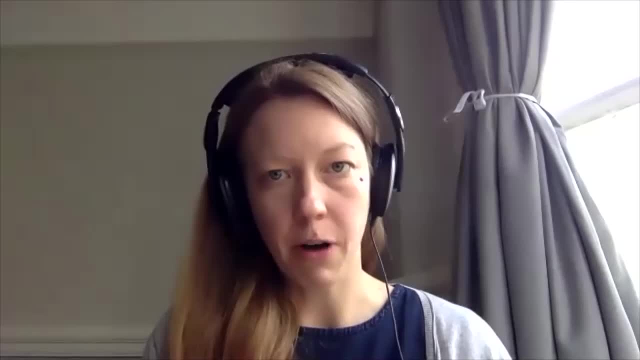 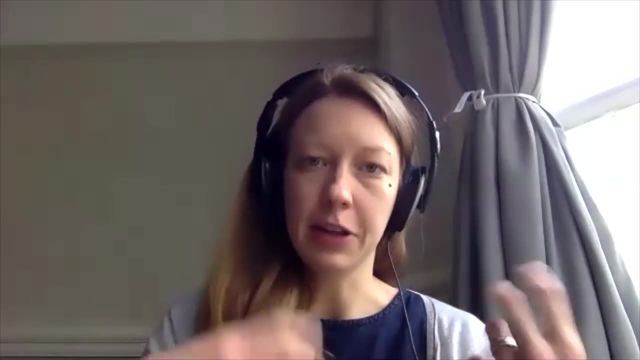 it's typically the gravity that's the important part. So I will code up the laws of gravity And then I can put all of this together and really study how a gas evolves under the gravity of a black hole and how the gas physics sort of evolve in this context. What we do is we build these very. 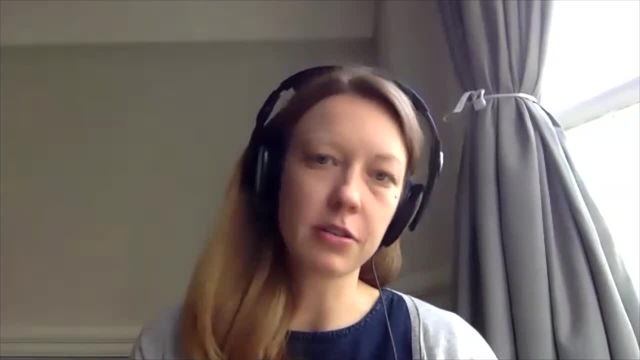 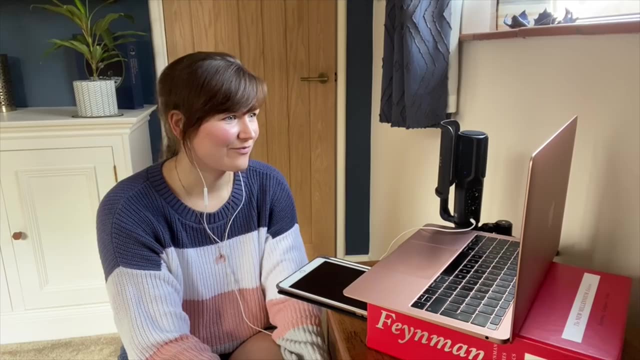 big codes that have all these different parts of the black hole, And then we have to think about what are the parts of physics in it. So I don't do all of this myself. A lot of these codes are the code I work with, for example, was started about 20 years ago or so, And there's a whole 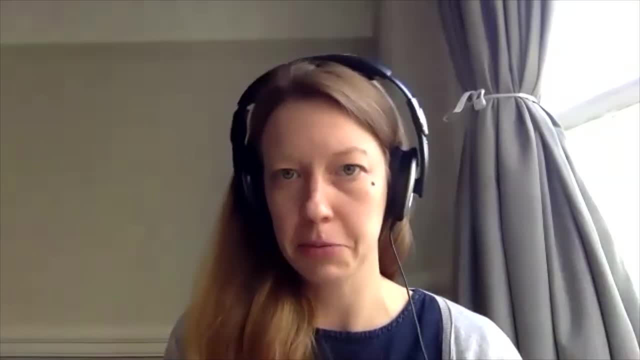 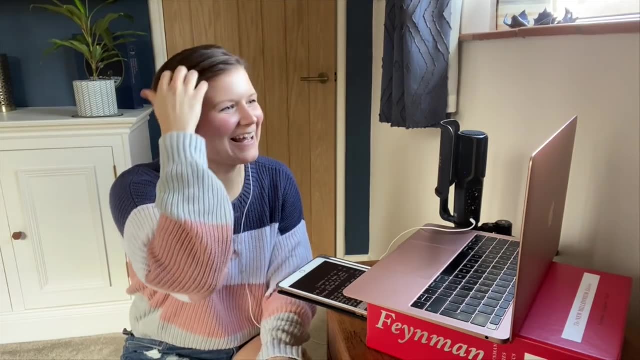 community working on it. Basically, we've sort of collectively built this incredible powerful software machinery to do these simulations. That's so cool that you leave your own little contribution as well, like in the history of the field, I guess even like students in 20. 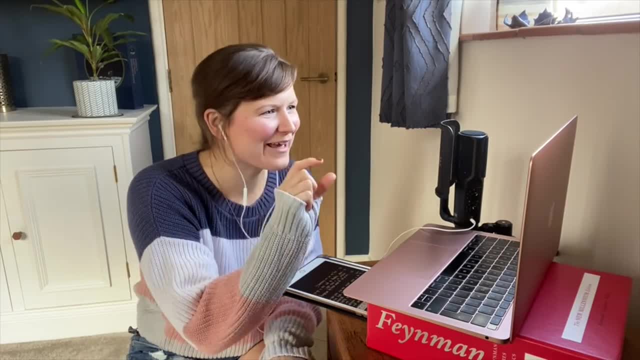 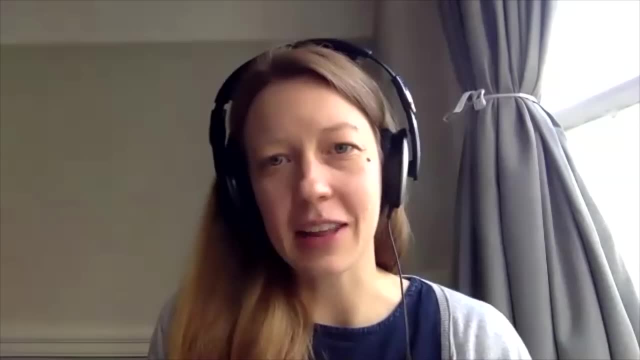 years time, or researchers in 20 years time might be using like a little bit that you added Right exactly, So you know if it goes well then and if that's still a phenomenon they're interested in at the time and that's relevant. 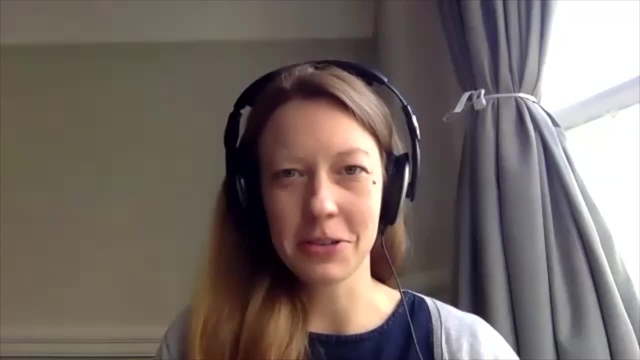 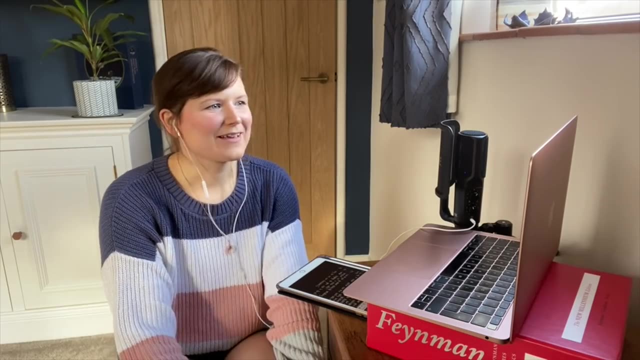 for their physics. they will just use my code, the bit I added, And so I do my own work, but I also contribute to the sort of future of the field in a sense. So what language do you actually use to code up like the laws of physics into this, Like what's the best one for this application? 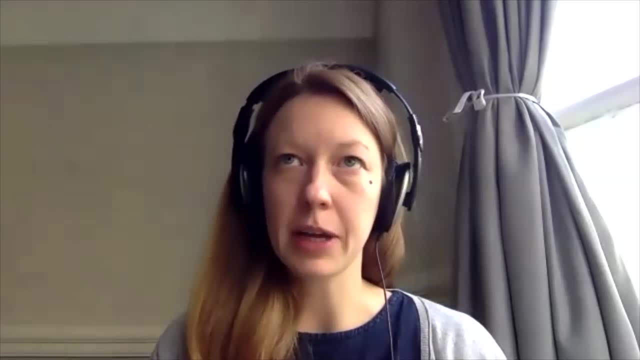 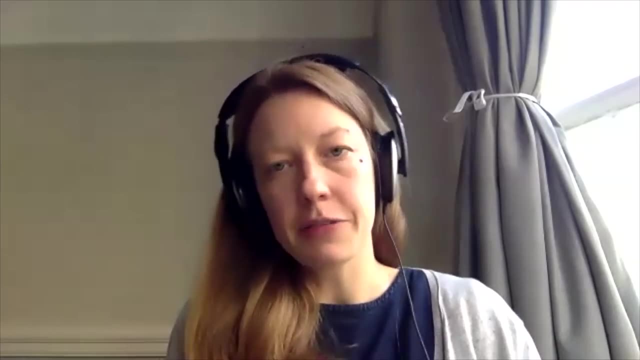 So it depends a little bit on which part of it. So really, with doing simulations, there's actually more like two very parallel things we have to do. So the first thing we have to actually do the simulation, and then we have to take the data produced by the simulation and sort of analyse. 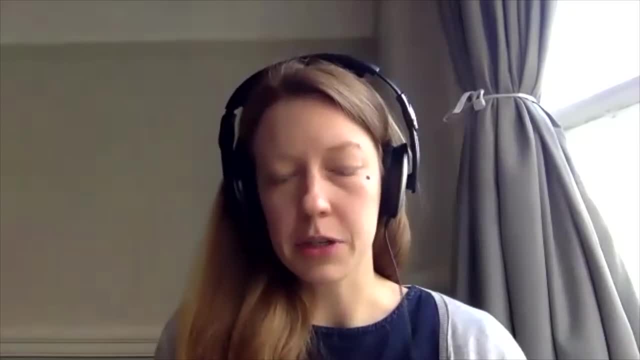 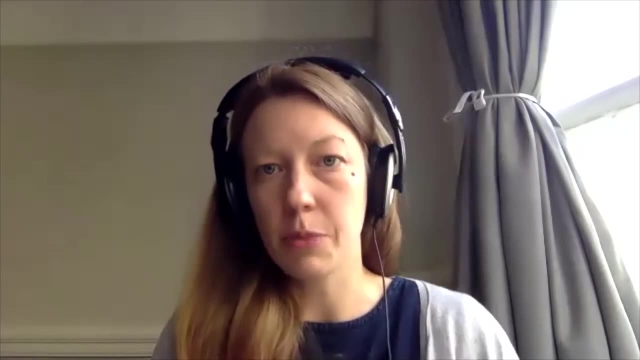 and visualise and study it, and we use two different coding languages for the two different purposes. So for actually running the simulations, this is what we call high-performance computing. So it's computationally very expensive. You need very big supercomputers to do it. 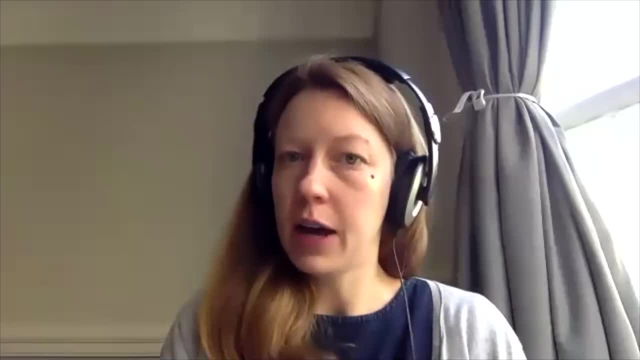 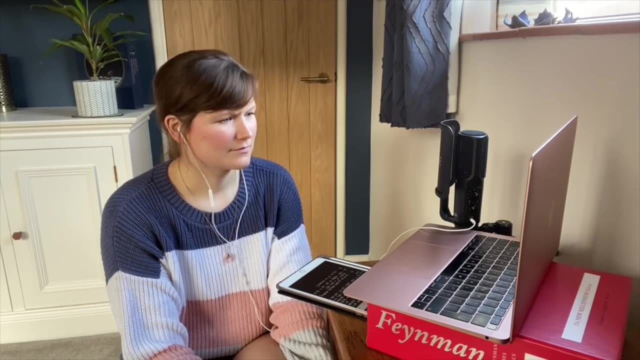 So the important thing here is to have a language that's efficient. So you know, any amount of computation time, energy we can save in this is good. So we tend to work with all the more formalised languages in a sense. So I personally use Fortran, for example. So these are ones that it's maybe a 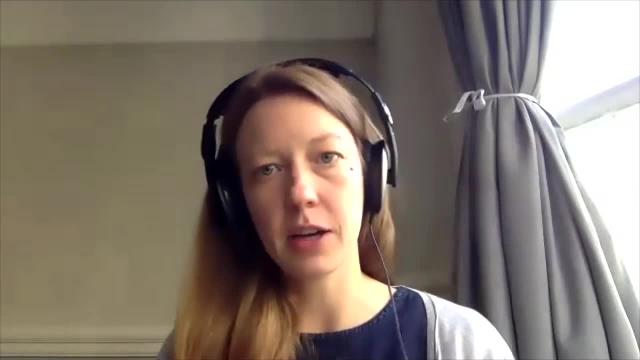 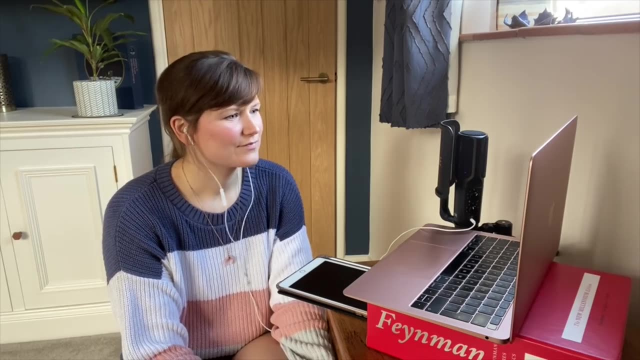 little more difficult to code. but because it's code we write once very carefully and then use many, many times, These sort of efficiency gains we get out of the language are really important and really worth it. So that's sort of the actual simulation code. But then, once we got all this, 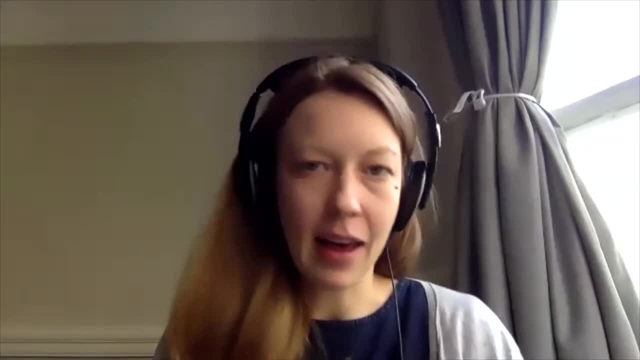 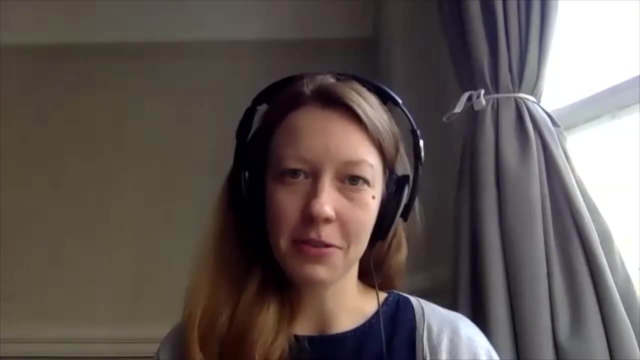 data. we need to go and look at it, analyze it, study it. you know, And for that I use Python, because the point there is that we want to write quick code. We want to have, you know, be able, something that's intuitive. I want to be able to put something together and you know, follow. 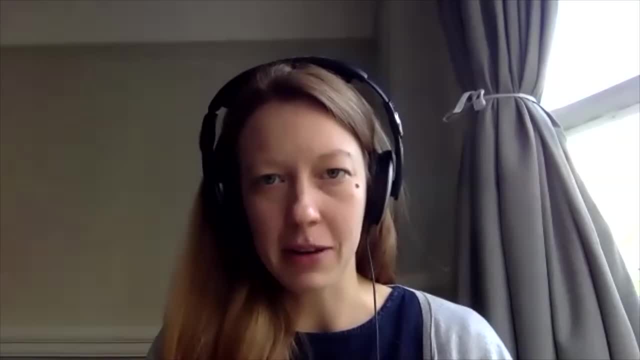 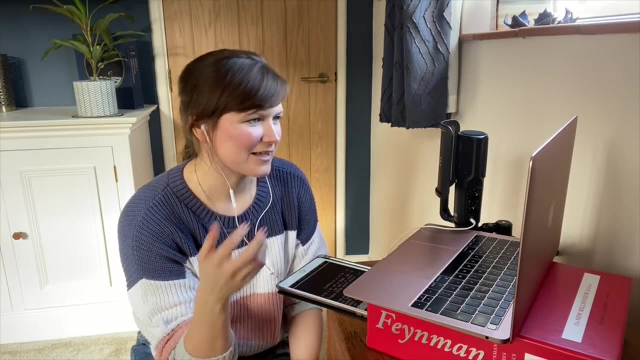 through on an idea really quickly, And I know you've talked about earlier, about Python a lot, So I think for the exact same reasons we use it for the analysis as well. I guess the big question, though, is: why do we actually run simulations Like? why are simulations so important in astrophysics? 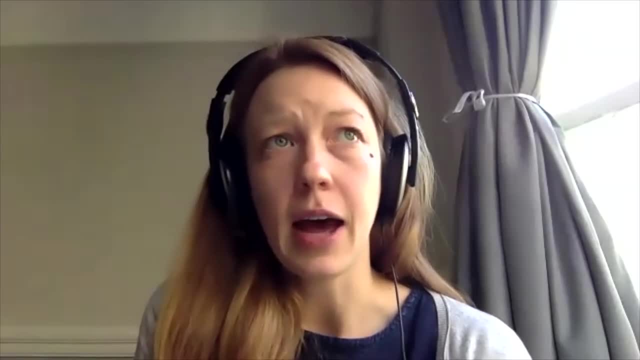 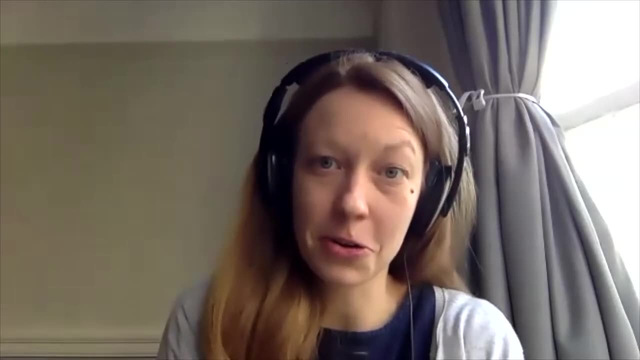 The reason simulations are so important is because in astrophysics we have a few very particular challenges in this sort of particular science. So one of them is that it's awfully hard to do experiments because you know there's only one universe, It's really big, The time scales over. 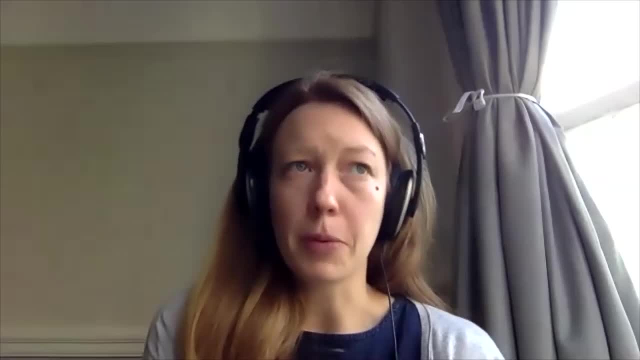 which you can do. experiments are really big So it's really hard to do experiments because things evolve incredibly long. So from an observational point of view, we often just get the sort of individual snapshots of objects, And the powerful thing about simulations is that it. 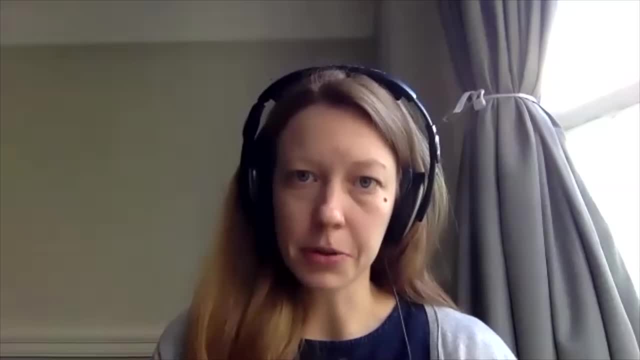 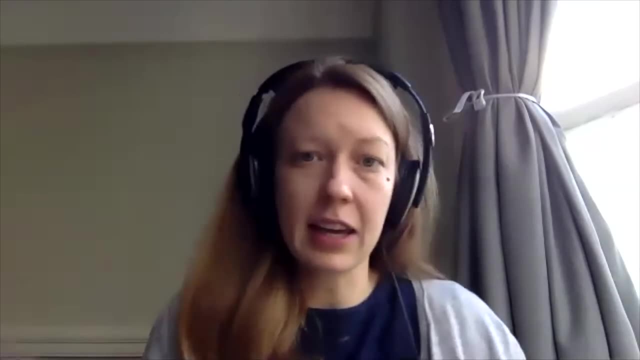 makes these big time scales and these big length scales very tractable, because we can essentially put together these simulations which you know. a big simulation would just look like a movie of an object evolving over giga years of time and you can watch it in five minutes. So, basically, 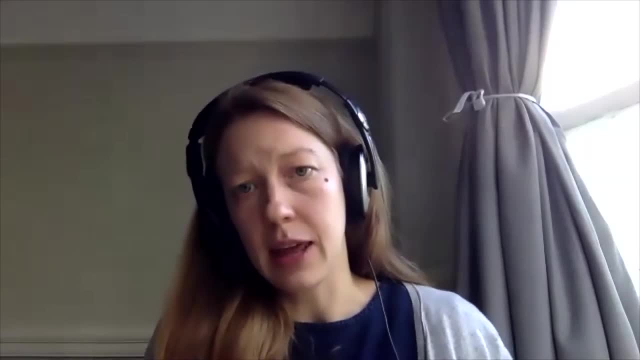 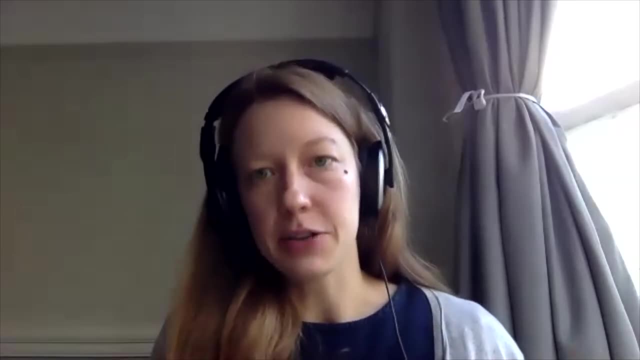 this gives us a chance to sort of build these evolution histories and then link that to the things that we think it should look like, like the observations, And that allows us to sort of test whether the physics we put in originally- what I talked about earlier- really is all the relevant. 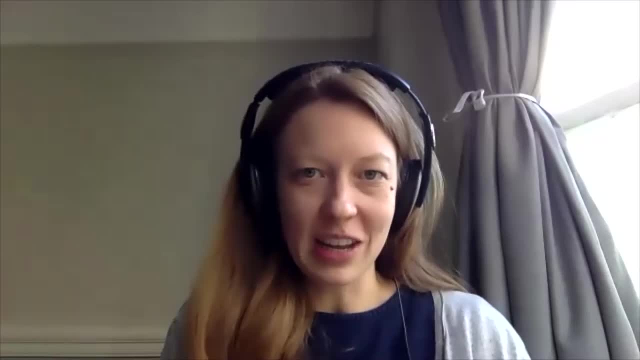 physics. If it looks like what we'd expect it to, then we think we've understood it. If it doesn't look like what we'd expect it to, then we have to go back and sort of, you know, go back and check. our understanding. What did we miss? What did we maybe misunderstand? Where could the sort of you know discrepancy come from? So really, they're a way to test our understanding but also to sort of you know, get full sort of long term evolution histories. 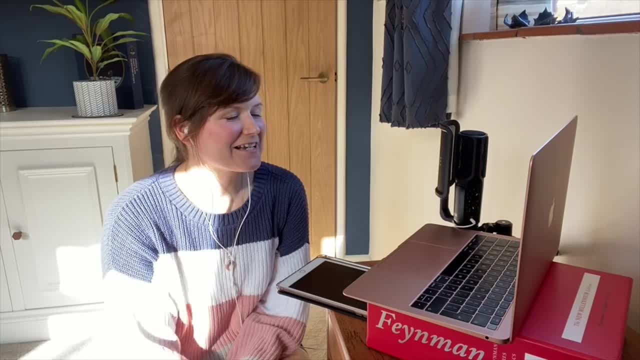 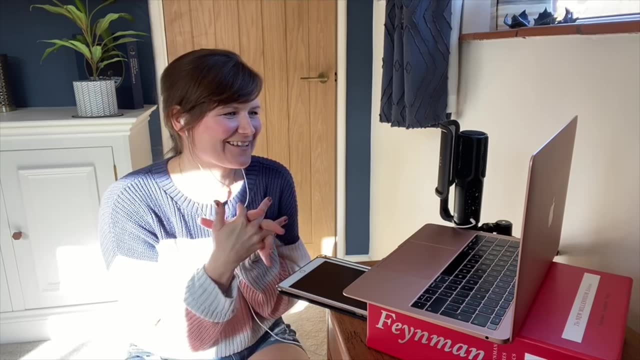 It's nice to know that everyone can like come together and work together to create something you know as like complex as simulating the entire universe, because I guess it feels overwhelming. Who was the first person that just like sat down and was like? 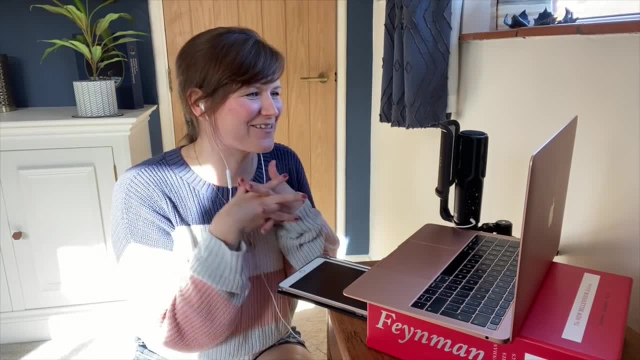 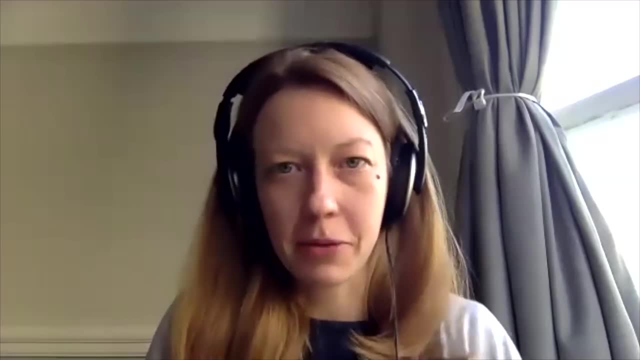 right time to start a simulation of the universe, Like that must have been. so, like you know where do you start. Yeah, I think it was somebody's PhD project. He's now a professor. well, the code I work with. he's now a professor in Zurich, So you know his. 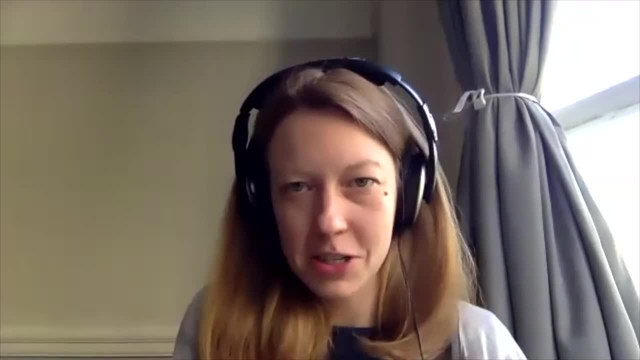 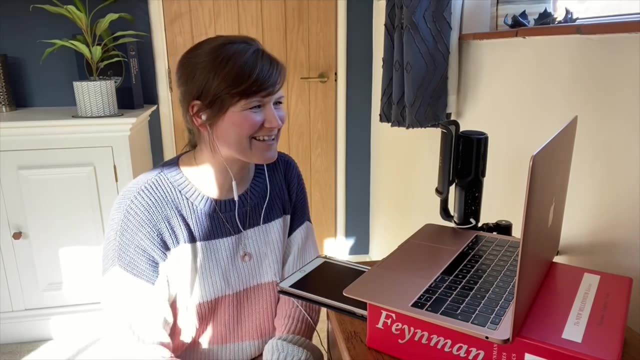 his entire career has been this code, And he started it. he published the original paper that said: here's a new code, And then people have been building on it ever since. That's so cool. Thanks, Riccarda, It was really great to speak to you. 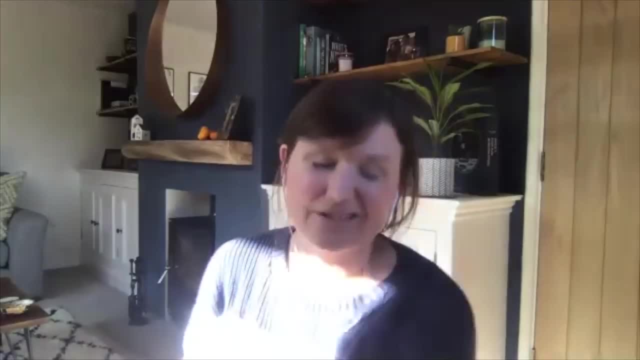 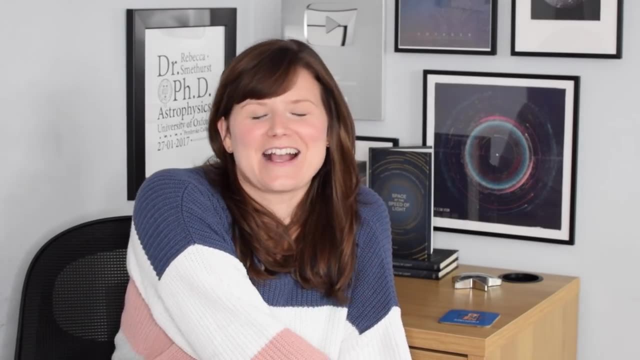 You're very welcome. If you want to hear more from my chat with Riccarda, I'm going to be posting the full, unedited version on my channel on Sunday, So keep an eye out for that. Thank you, Riccarda, for our nice little catch up there. I hope that helped you realize. 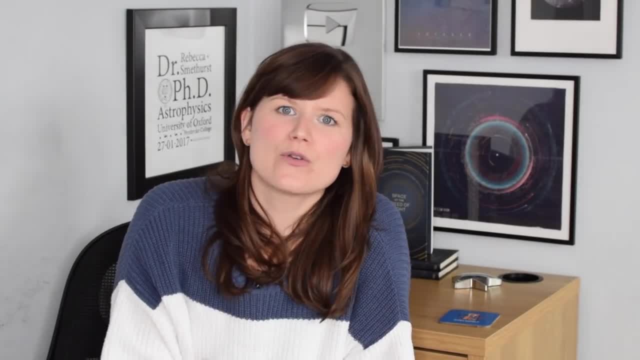 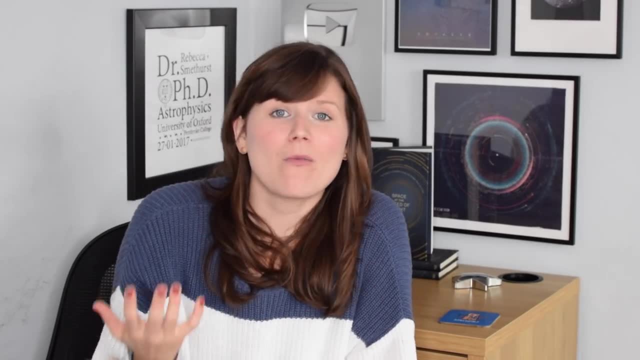 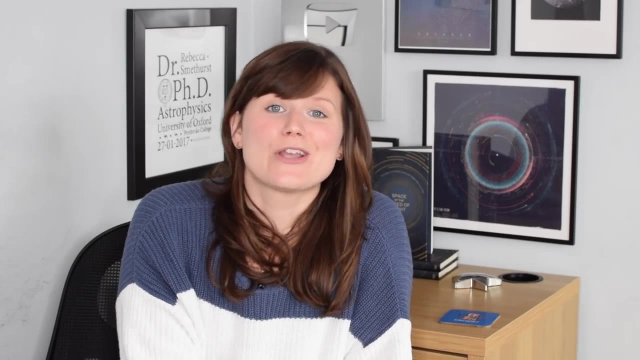 how astrophysicists like me and like Riccarda use code day to day in our research And after that. well, you might be quite inspired and you might want to learn to code yourself and not really know how to start. Well, I always find the best way is to learn by doing which brings. 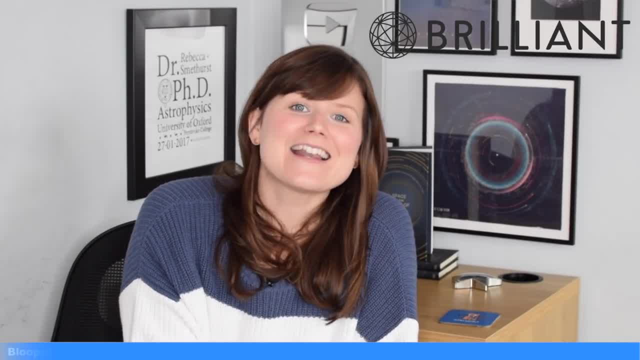 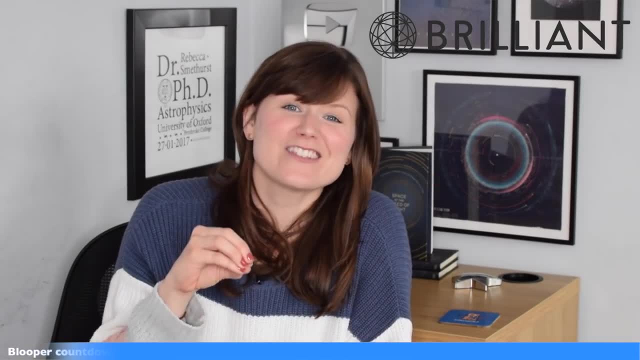 us to this week's video sponsor, Brilliant. Brilliant is a problem solving website with lots of interactive courses that break down problems into easy to understand chunks that are really fun too. They have courses on a huge range of science and maths topics, but I wanted